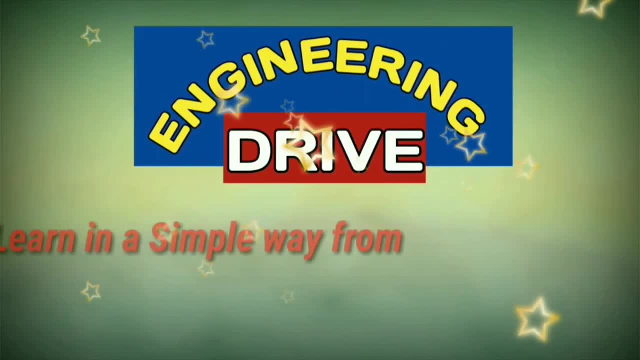 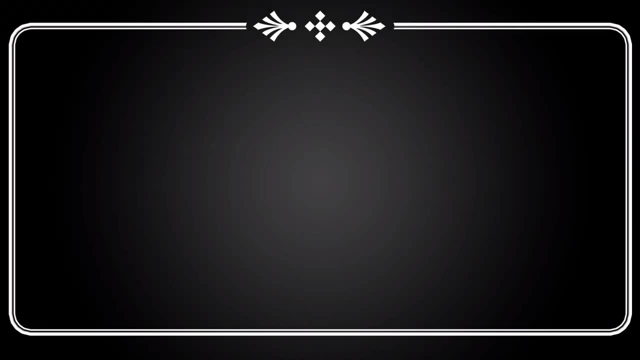 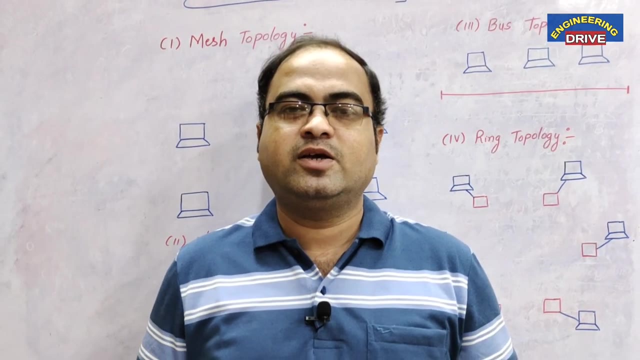 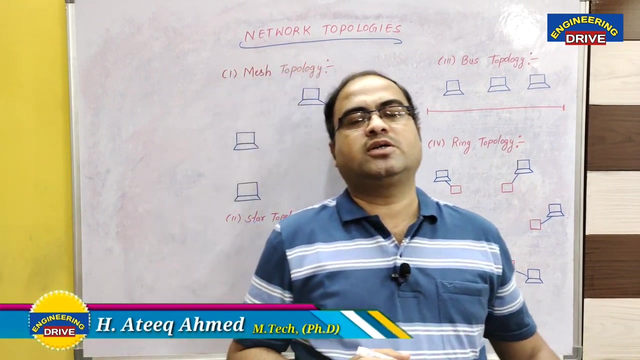 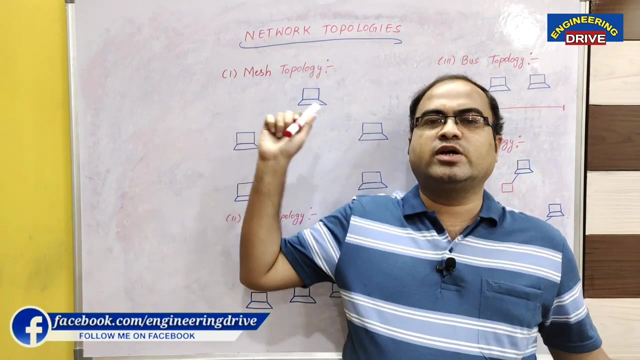 Hi, everybody, hope you are all fine. This is Atiq. I welcome all of you to our YouTube channel, Engineering Drive. Let us discuss about the various ways in which a network can be organized. We call this topic as network topologies. Topologies are nothing but a structure. 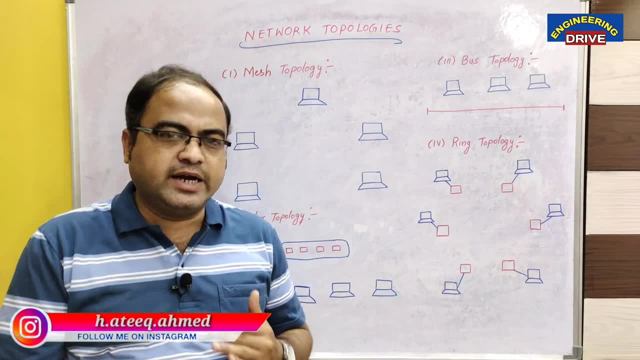 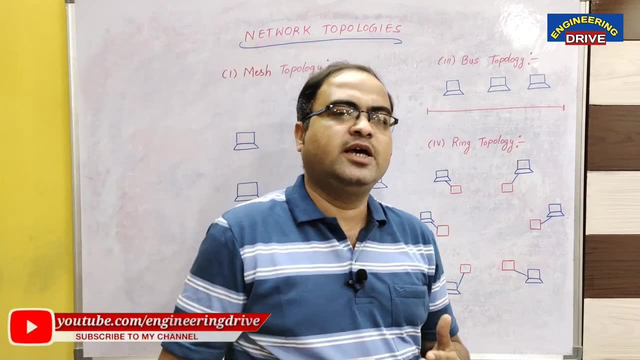 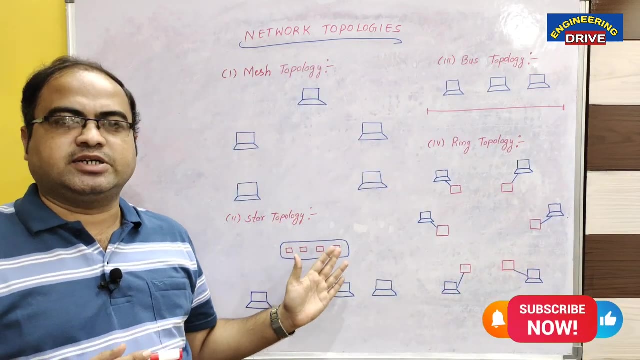 or we can say: the way a network is organized is nothing but the network topologies. So what are the different types or what are the different ways in which a network is organized? So I am going to discuss each and everything in detail with the diagrammatic illustration. So, dear, 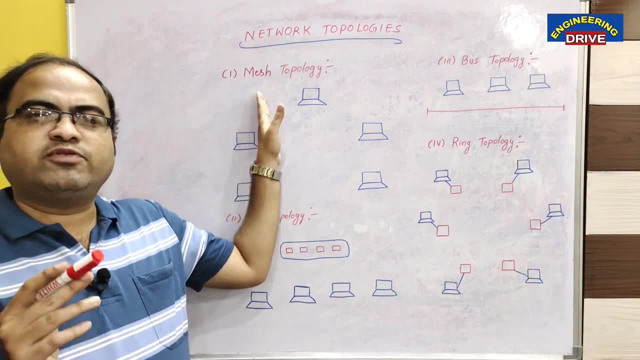 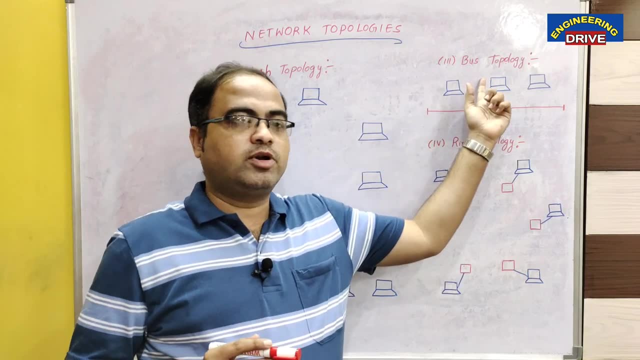 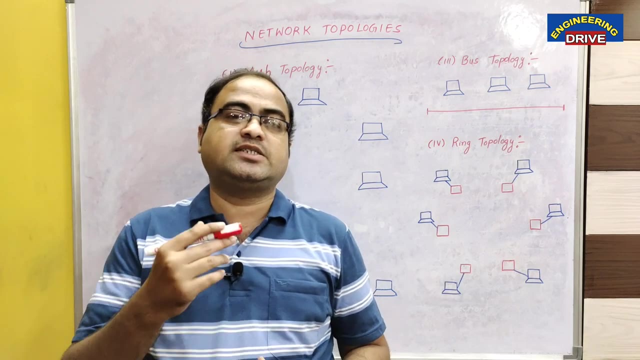 students. you can see here there are four types of network topologies supported. Number one: mesh topology, star topology, bus topology and ring topology. This concept is very, very important for both competitive exams as well as in external exams for the students because 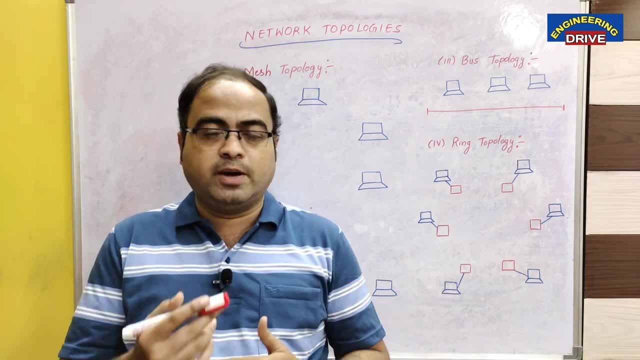 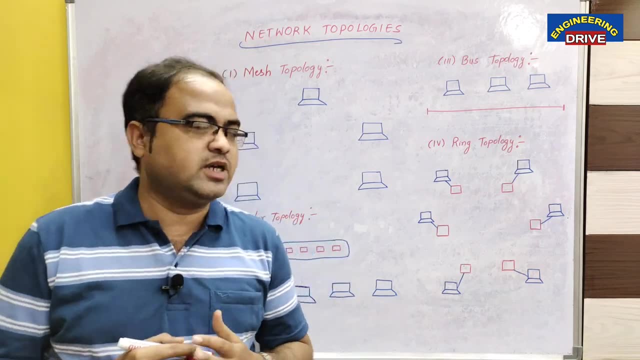 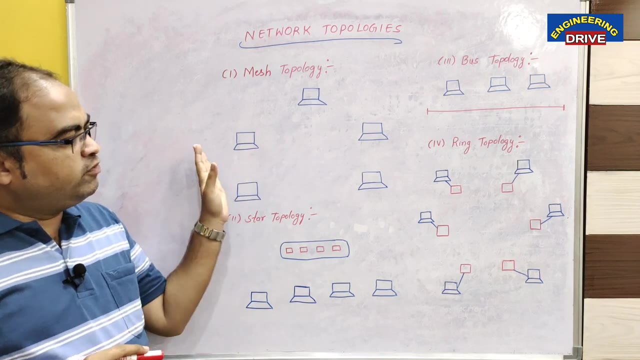 many questions will come from this topic in the form of bits, as well as this question, because I believe that you are going to give a full focus on these types of topologies in a network. Now, first of all, before directly going to these four types of network topologies. 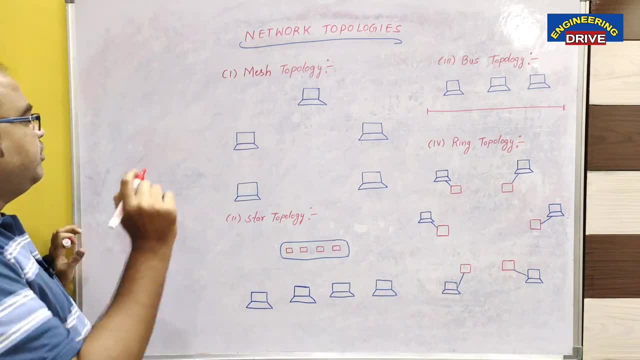 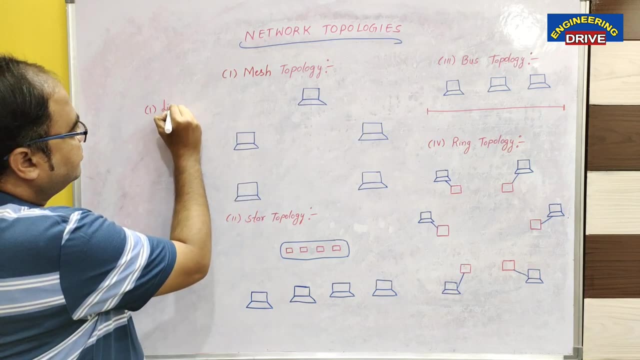 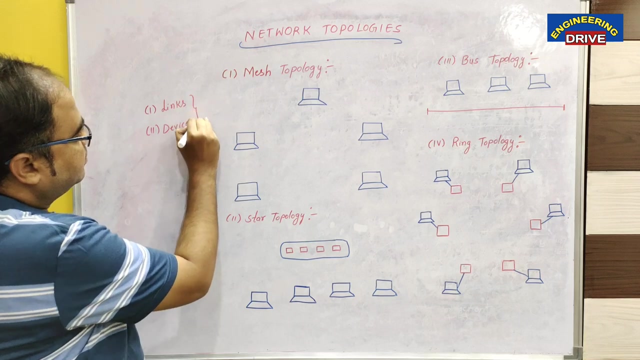 we should know that in a network, the two important things that we need to understand and need to remember is: one is the links and the second one are the devices. Okay, so let us look at this. So here, links are used for connection and devices are the individual. 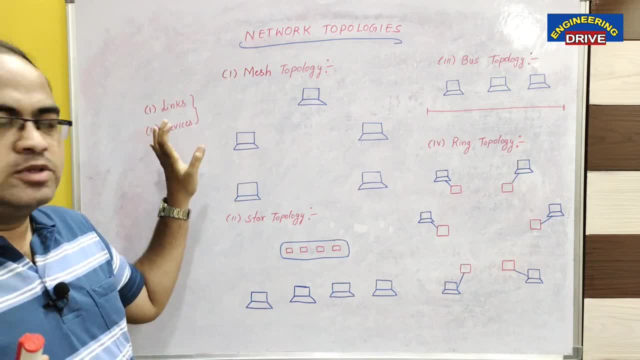 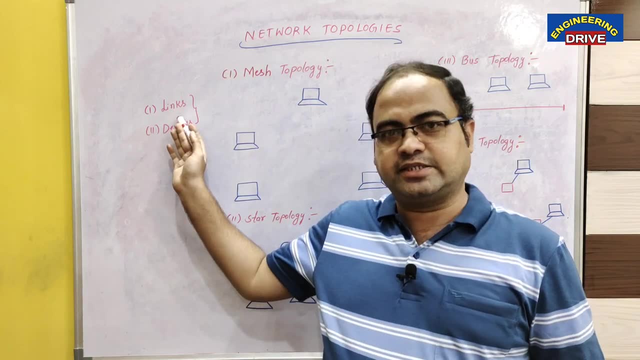 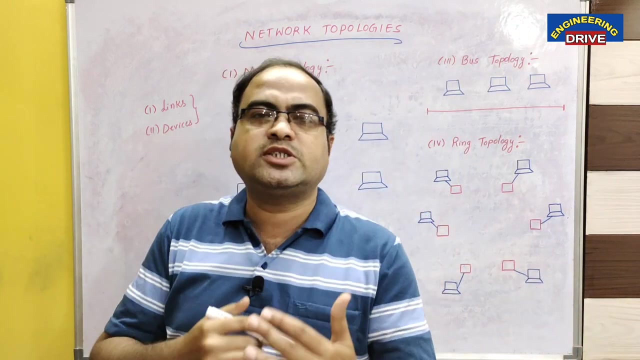 entities. So these devices are connected with the links. So this is the overall structure of a network. A network is organized by using devices and links. We know that Now. how these devices and links are organized in a network, network topologies will give the answer for. 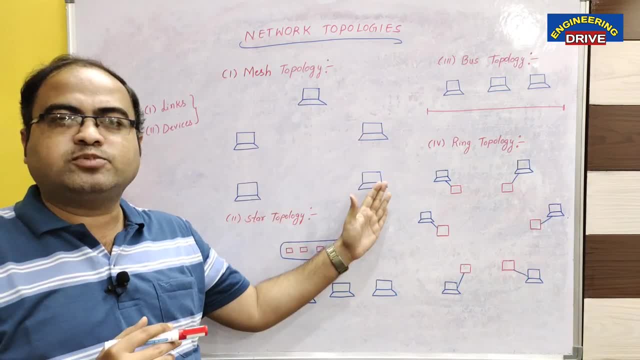 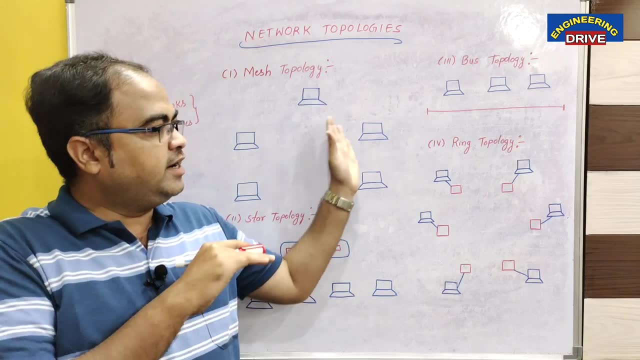 us. So for that, let us discuss about these four types of network topologies. to know how a network is linked with a network. So what are the four types of network topologies is laid out and what are the different ways in which the devices are connected by using links. 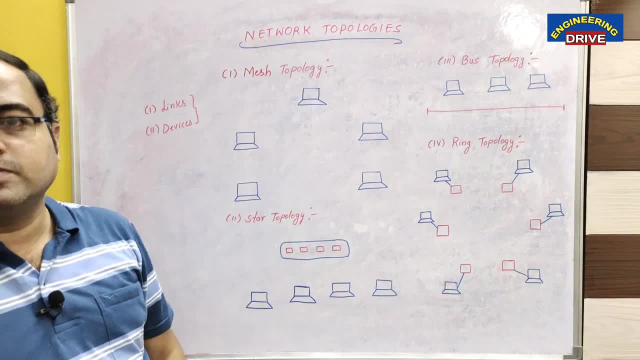 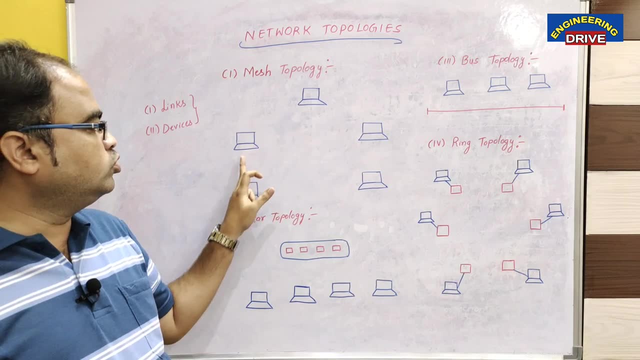 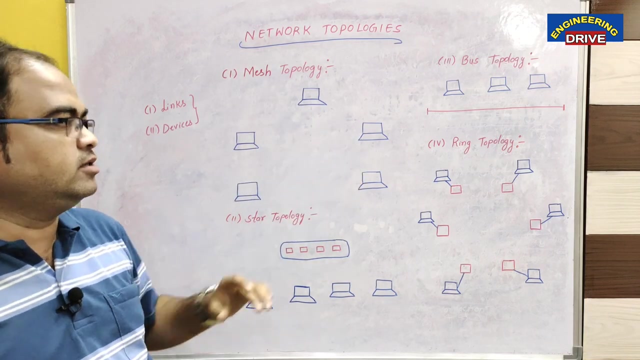 So let us discuss the first one now: mesh topology. Okay, in mesh topology, let us consider: five devices are there now here? How many devices? Five? One, two, three, four, five. These are the five devices Now in mesh topology, how these five devices are connected with each other. 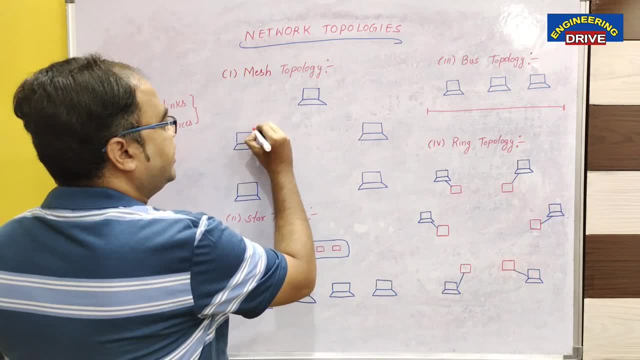 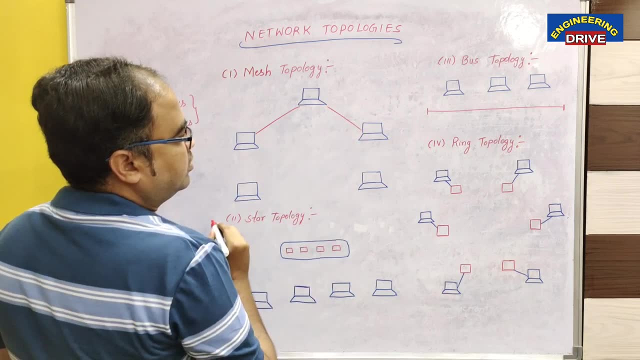 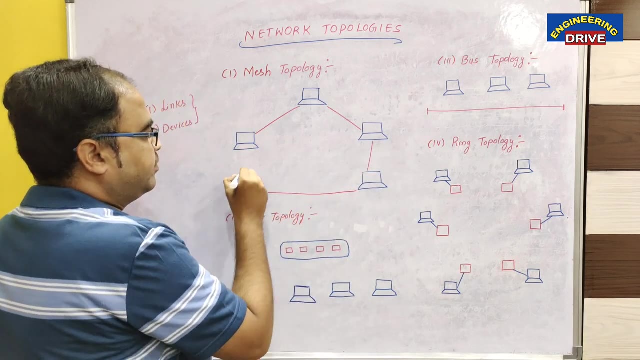 Every device will have a dedicated point-to-point link here. For example, from this device to this device, from this device to device number two. from here it will have one more connection and from here it will have one dedicated point-to-point link. and here also one dedicated. 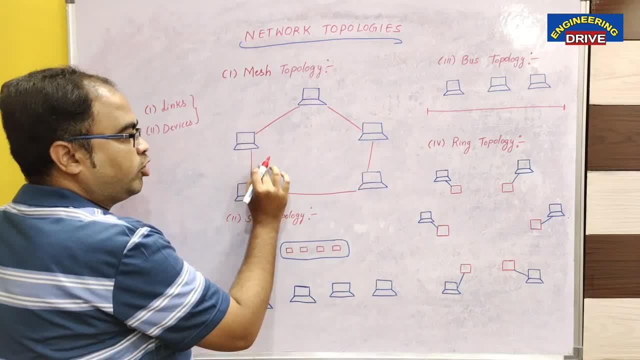 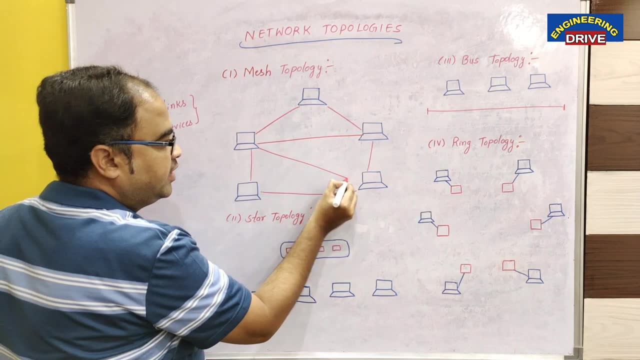 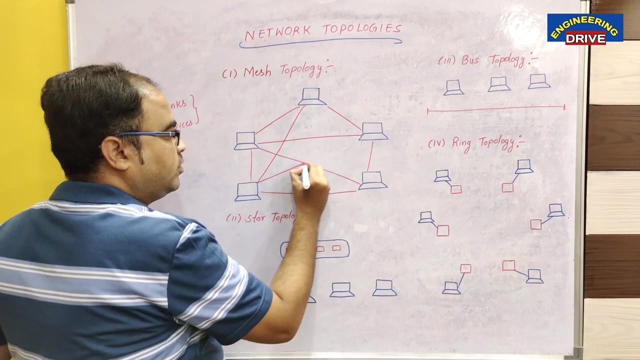 point-to-point link. So every device will have one dedicated point-to-point link and again, this device will have a dedicated point-to-point link. From this, it will have a dedicated point-to-point link. Similarly, this device will have one dedicated point-to-point link and this device 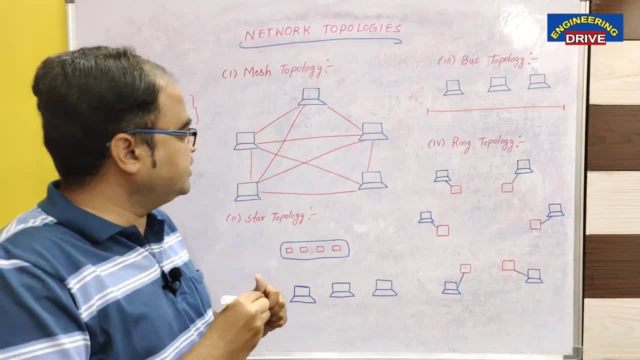 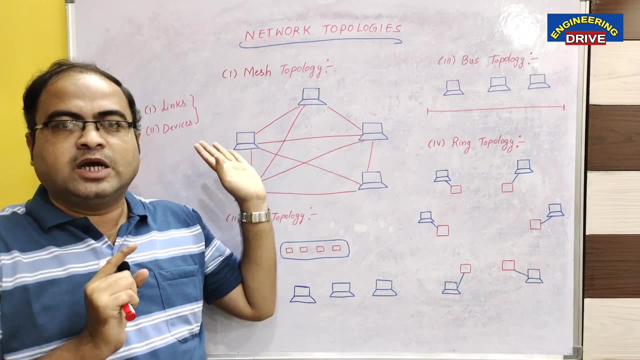 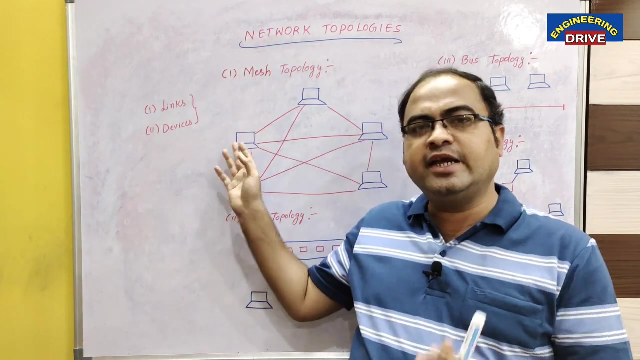 will have one dedicated point-to-point link. So, dear students, you can see here every device is having one point-to-point link to another device, which means, in mesh topology, if a device want to communicate with another device easily, any device can communicate with any other device. 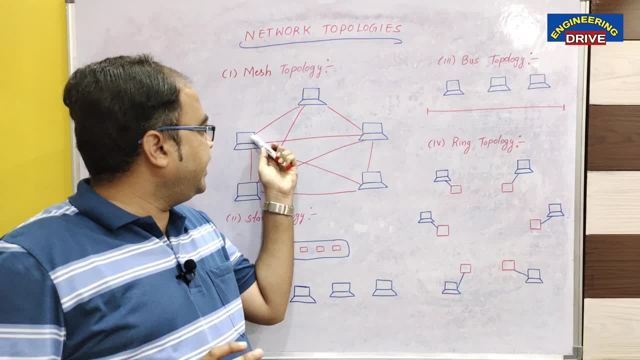 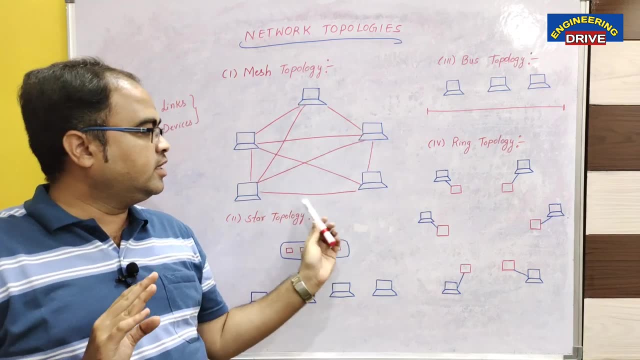 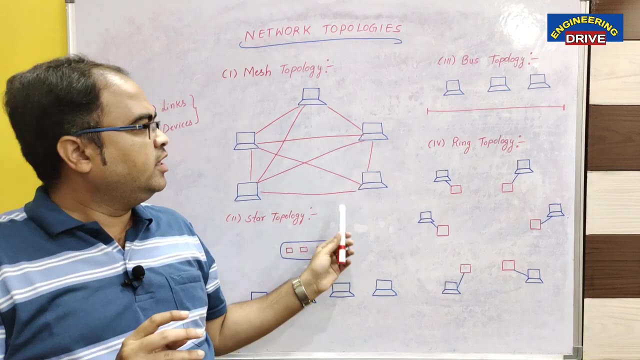 Why it is possible, Because of a separate connection will be available between them, So easily they can communicate with each other. This is how mesh topology structure will look like. Is it right Now? the biggest advantage of mesh topology is if any device failed, if any device is not working properly. 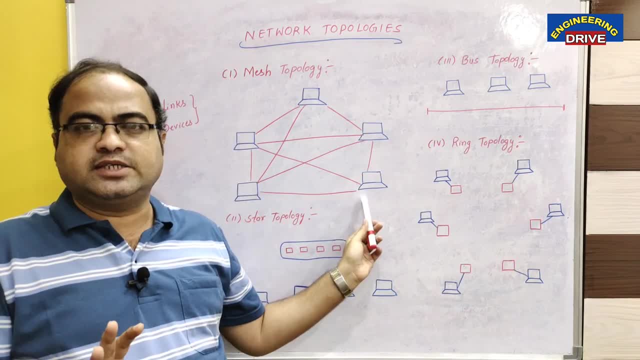 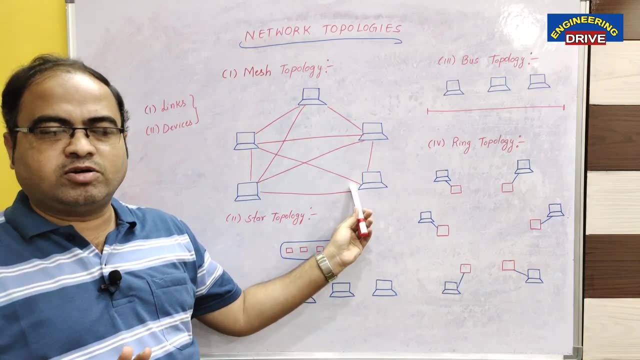 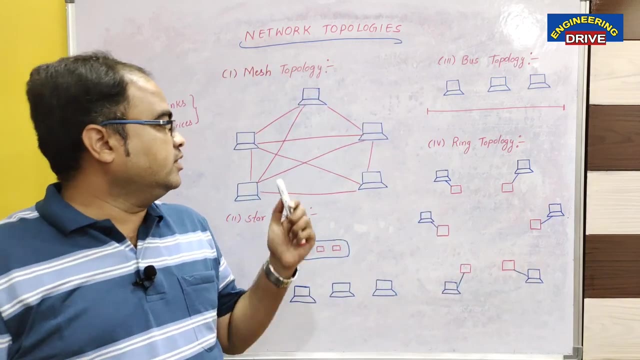 then it does not have the impact on remaining devices, because remaining devices still, they can communicate with each other because they are having the respective links, Is it right or not? And mesh topology is one of the reliable topologies on which we can depend. The big advantage of mesh topology is less chances of failure, and it will have. 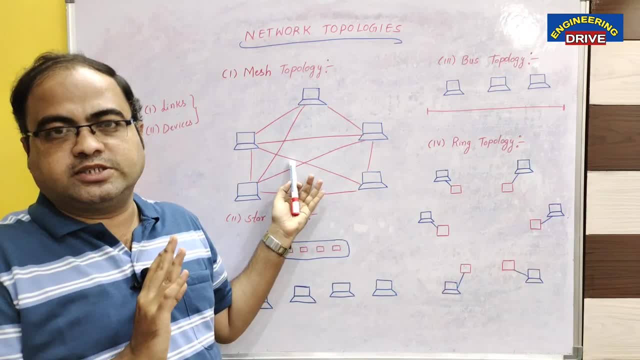 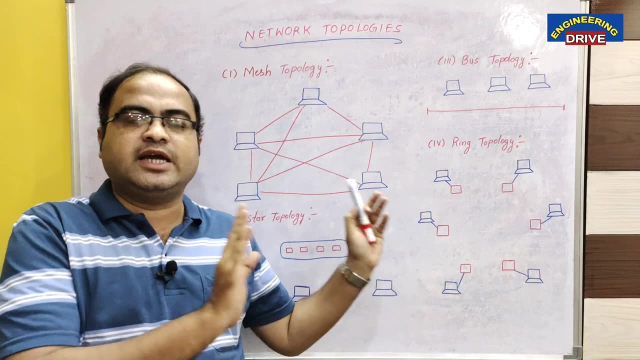 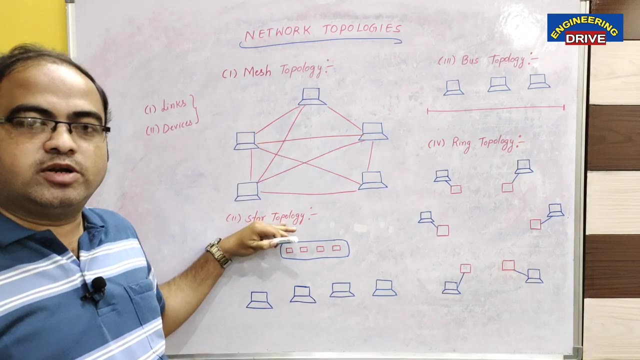 this topology will be much more reliable compared to other topologies, Is it right? And because of this dedicated point-to-point connection easily, any device can communicate with any other device without any problem. This is how mesh topology works. Now coming to the second type of topology, that is, star topology. So in star topology, 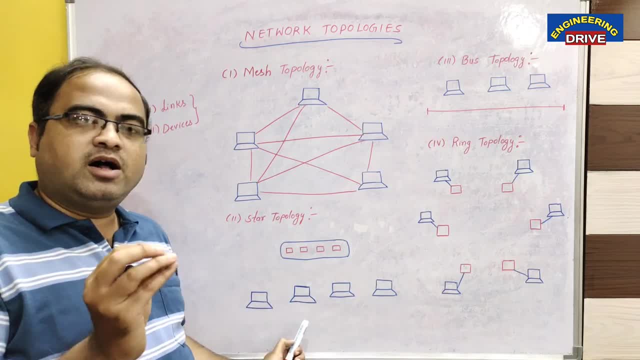 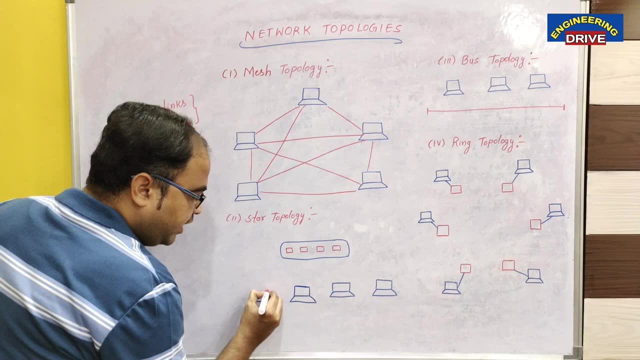 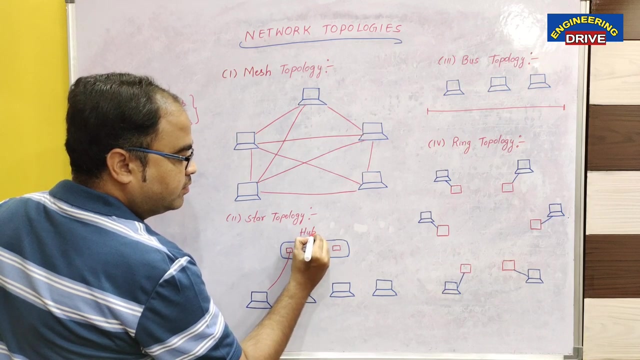 also, there are devices, and all these devices have dedicated point-to-point link. But what is the difference? you know, This device will have a dedicated point-to-point link to one more device. We call this device as hub. This hub acts as a central controller, Central. 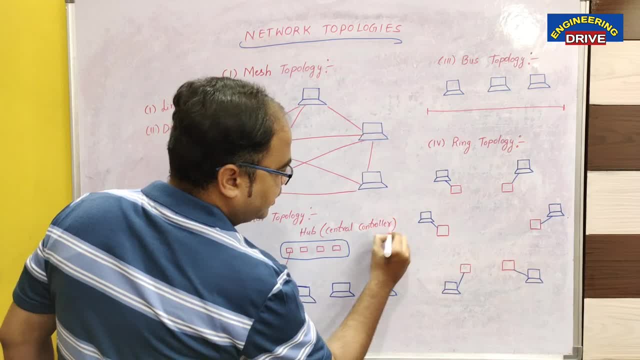 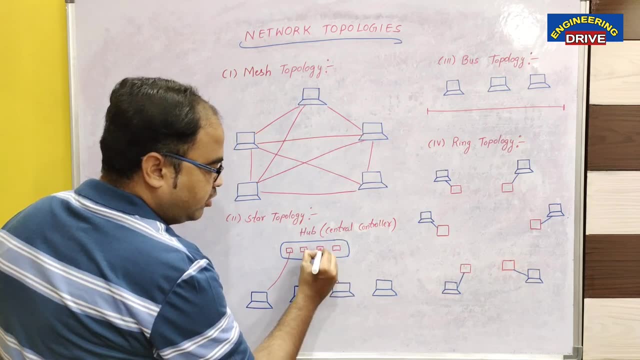 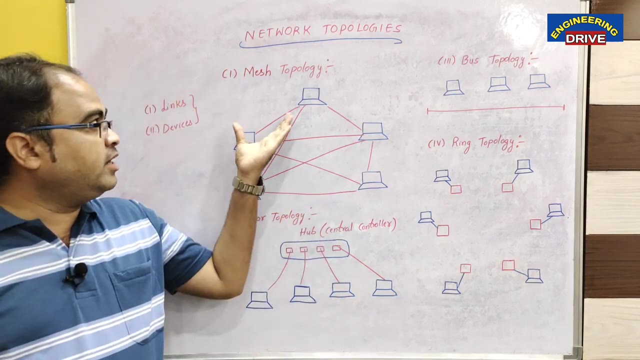 controller. So again, this device number two will have a dedicated point-to-point link to hub. Here also it will have dedicated point-to-point link to hub. Four devices will have dedicated point-to-point link to hub. Now you can see here compared with mesh topology in star topology. 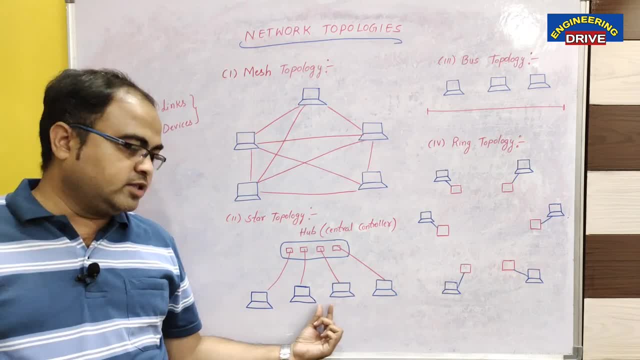 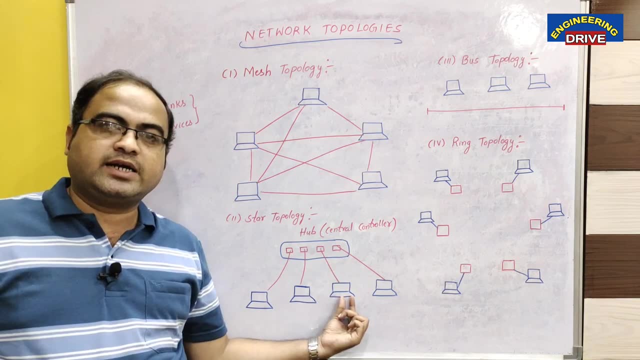 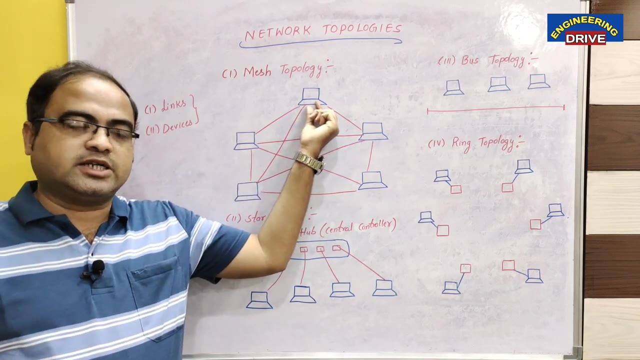 devices. they do not have connections among themselves. You can see here: first device does not have direct connection with device. second: Second device does not have direct connection to device. number three: Unlike in mesh topologies, we can see here: every device will have dedicated point-to-point connection Now, instead of 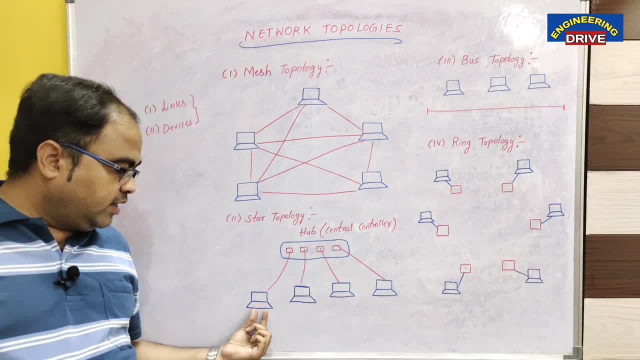 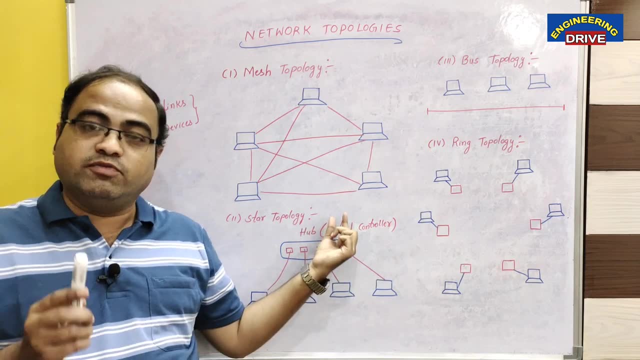 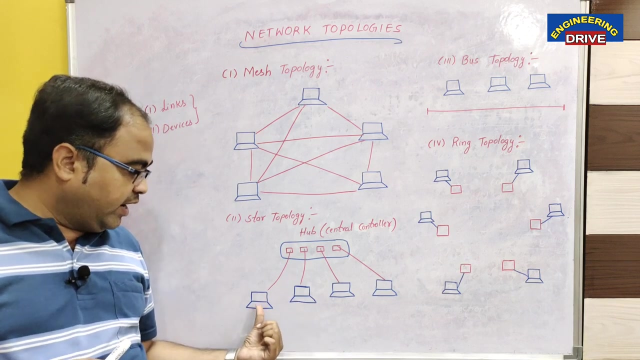 a dedicated point-to-point connection among themselves. every device will have a point-to-point connection to a hub which acts as a central controller. Which means, if device one want to communicate with device number two, then what device one should do? Device one should. 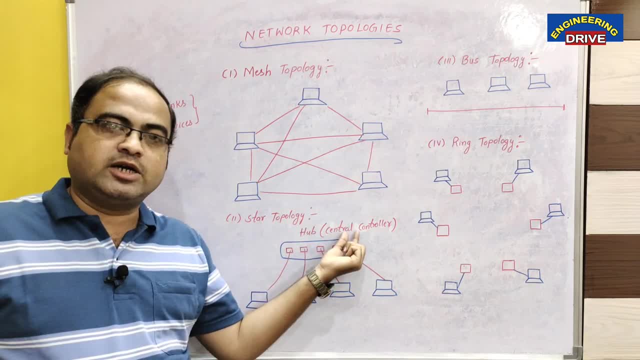 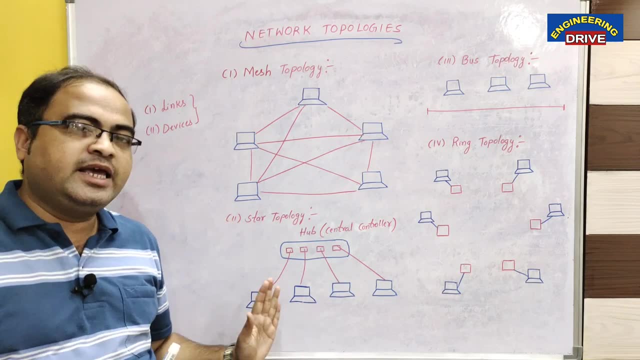 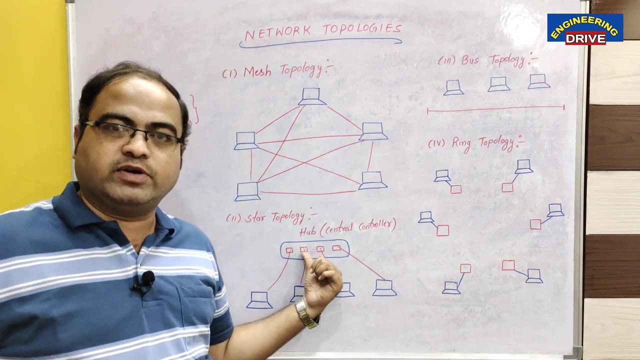 send the request first to hub, which is a central controller, And then hub will transfer the request to the device number two, Which means anything if a device want to communicate with any other device, compulsory the request should go to the hub first. That is a central. 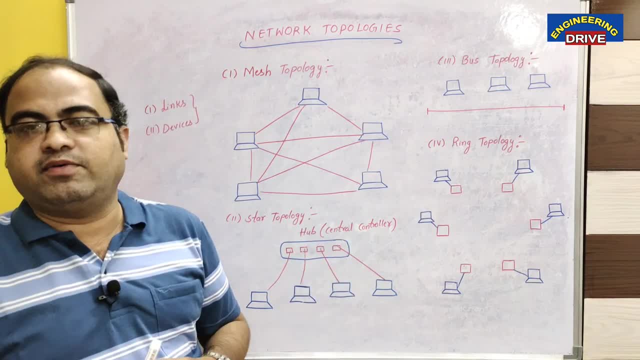 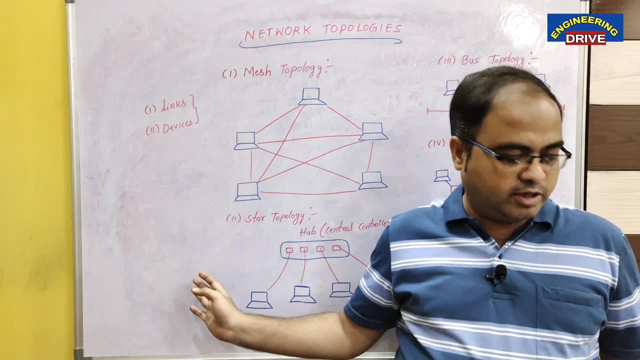 controller. From central controller it should go to the other devices. So the main difference, in a simple words I can tell, between mesh topology and star topologies. In mesh topology there is no concept of any hub or central controller. here, All the 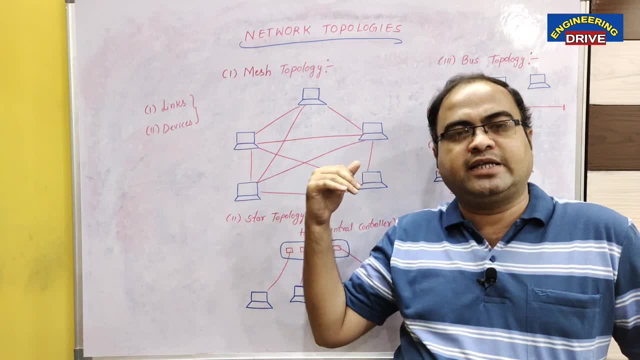 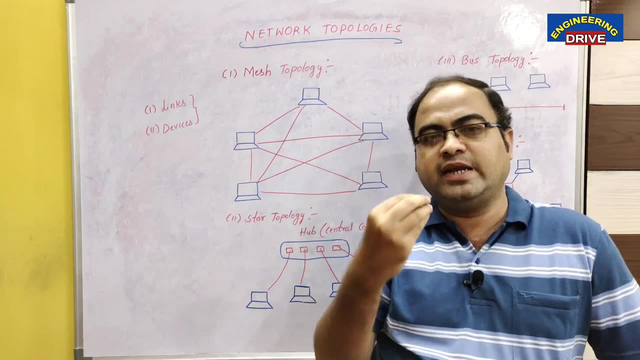 devices are themselves boss here. They can take their own decision and they can transmit the data without any problem. But in star topology if any device want to perform any type of communication, then that request should go to the central controller, which is a hub. 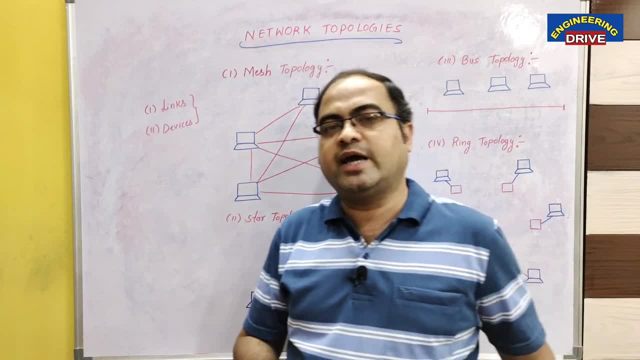 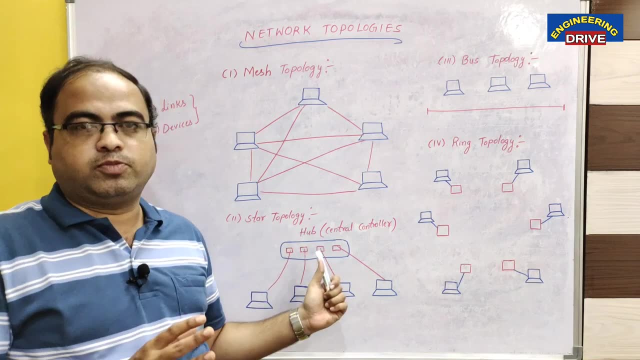 And from hub it should go to the devices. So in this way, what happened? The communication process can be monitored and it can be organized Subtitles by the Amaraorg community. That is one of the advantages of star topology, Is it okay? 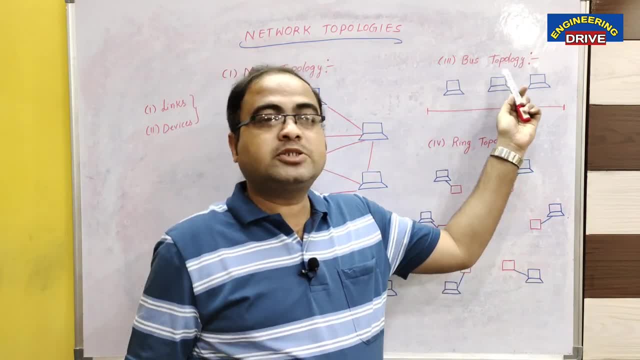 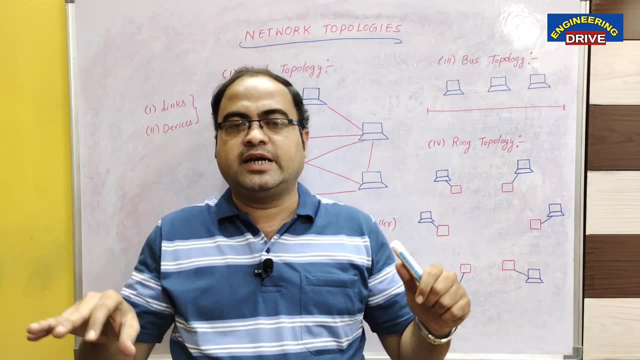 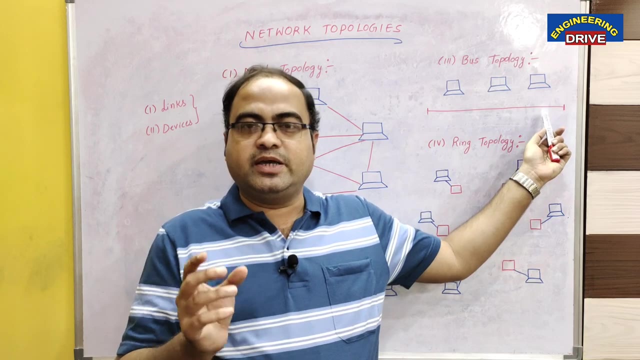 Next, coming to the third topology, which is bus topology, and it is the oldest of all these four topologies. This is the first way in which the networks are organized. What is that bus topology? In bus topology, what happened? A single link will be shared among 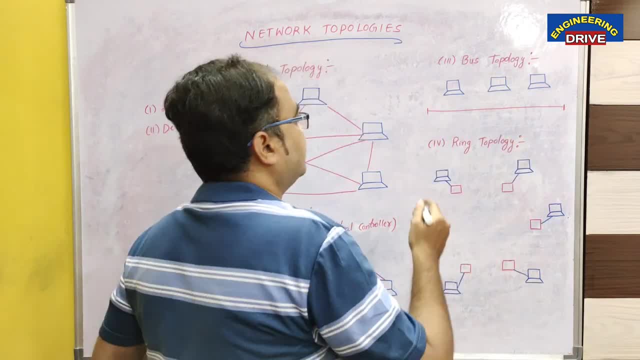 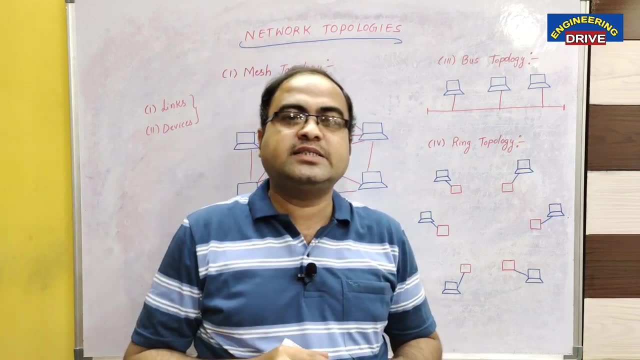 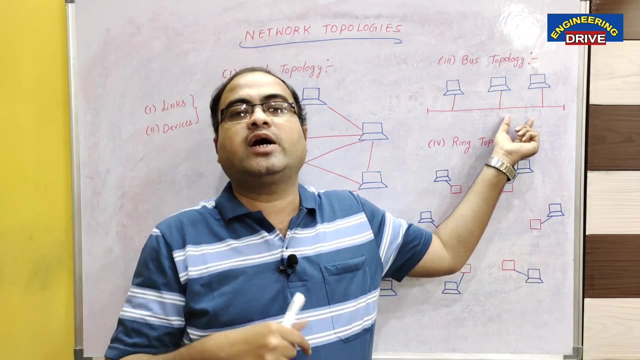 multiple devices. We can see here, this is a link and it will be shared among multiple devices And all these devices, they can communicate with each other by using this dedicated link, either in a timeshade fashion or in a spatial fashion. You know what is the meaning of timeshade? 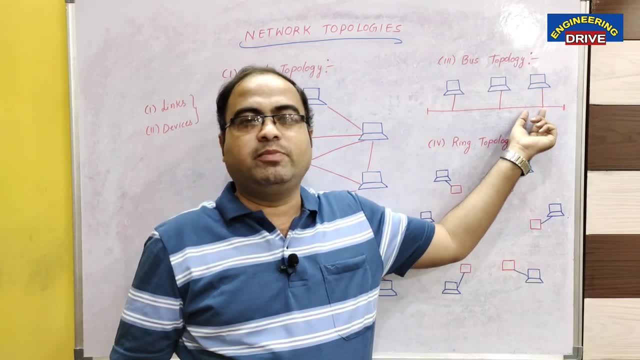 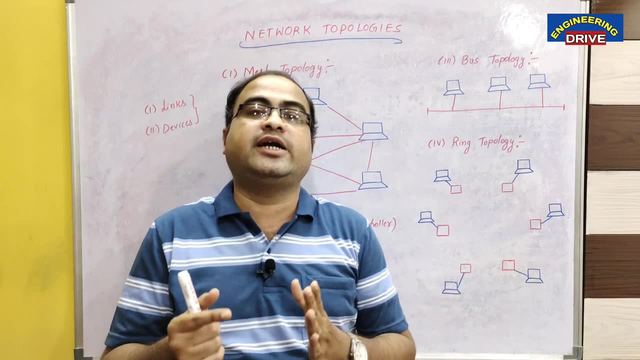 If two devices are communicating with each other, then third device will be ideal. If first and third device is communicating with each other, then device two will be ideal. This is known as timeshade manner, And there is one more way in which the devices can communicate. 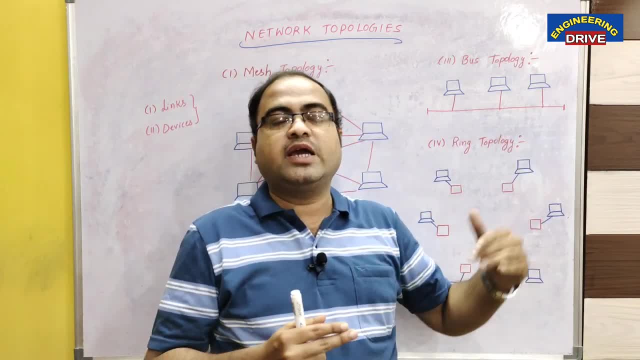 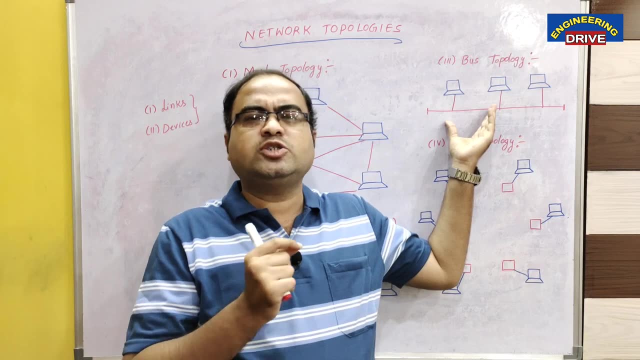 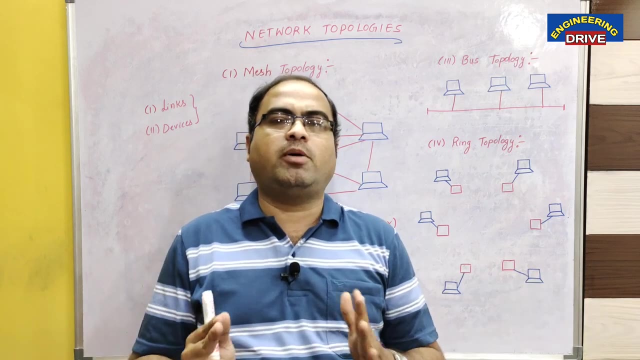 with each other is by sharing the bandwidth of the link. We can call it as spatial connection. So by using this also, the devices can communicate. The big advantage of this bus topology is it is very less expensive to implement. It does not require a huge or complex cabling, and 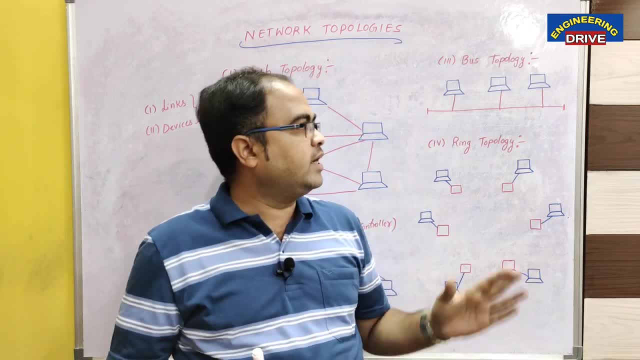 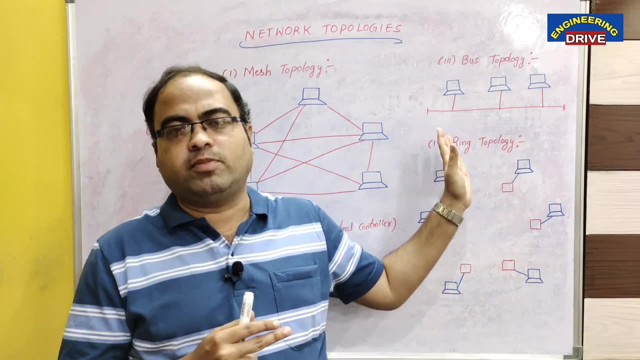 the setup can be implemented very fast, But the drawback is multiple devices. they cannot communicate simultaneously here in bus topology, And it is the oldest form of communication. All these four topologies, And then comes the fourth topology that I am going to discuss. 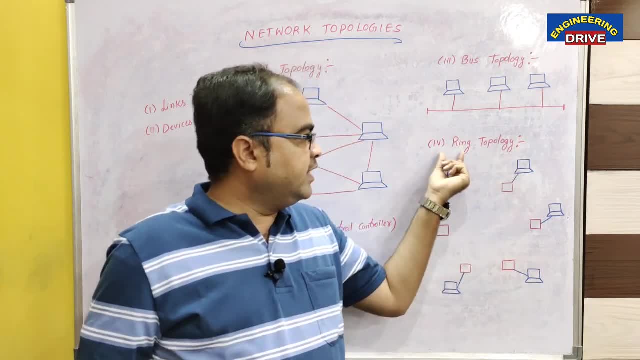 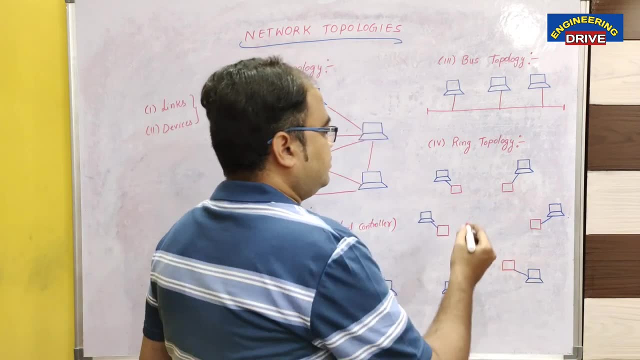 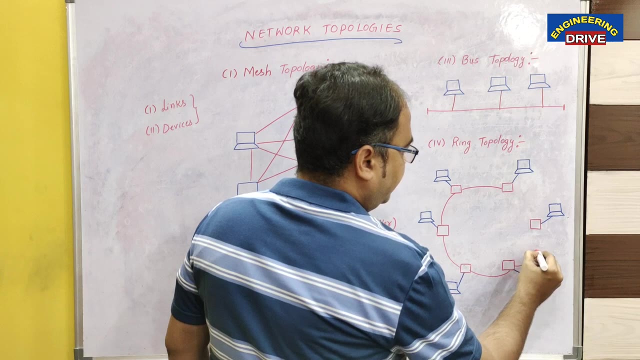 at last now, which is a ring topology In the name itself: answer ring. here The devices are laid out in a ring fashion, So you can see here, So all these devices, they are connected with each other in a circular manner in the form of a link, in the form of a cycle. 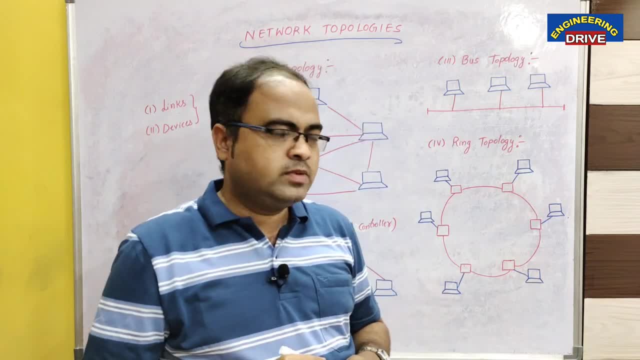 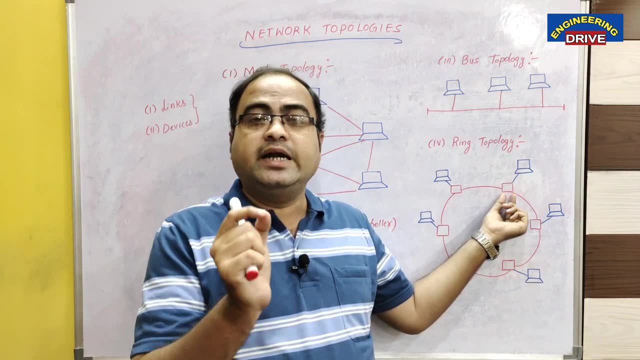 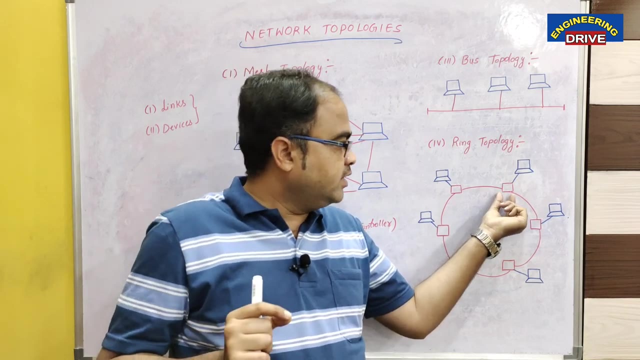 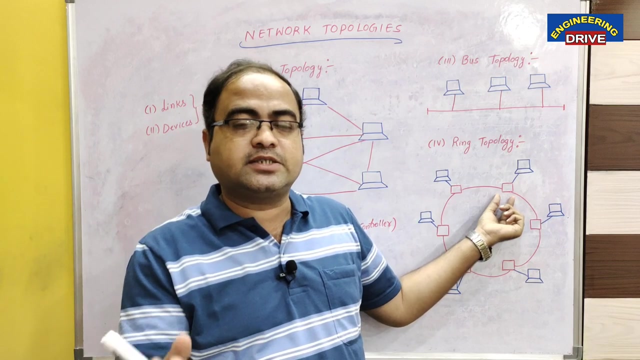 or we can call it a form of a ringer. Now, in ring topology, every device has a dedicated point-to-point link with its neighboring devices. Very, very important point, Dear students. you can see here, Let us say: this is my device. This device will have a dedicated point-to-point link to its neighboring devices. 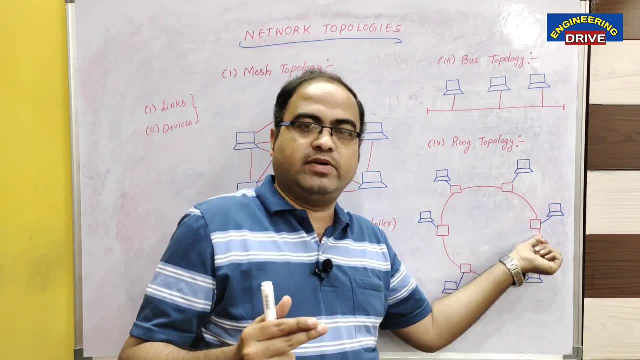 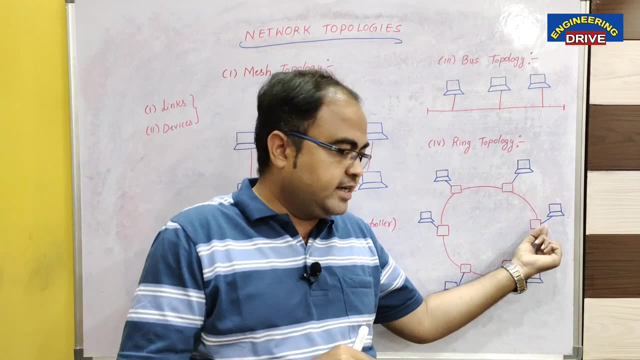 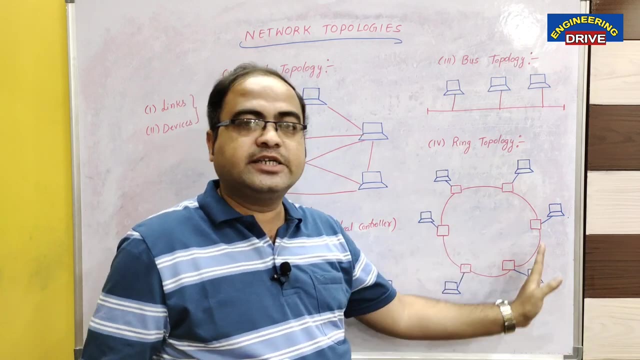 What is the meaning of neighboring here? Left side and right side device. Similarly, let us take this device. This device will have a dedicated point-to-point link to its left side neighboring device and then its right side neighboring device, like this: Okay, And this type of connection forms a ring structure. 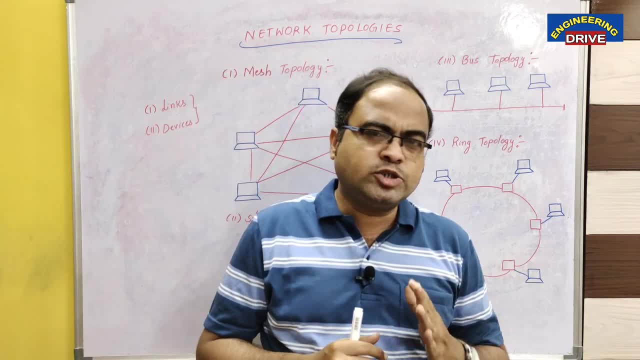 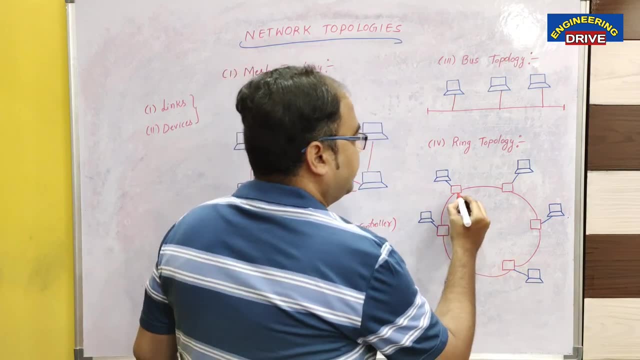 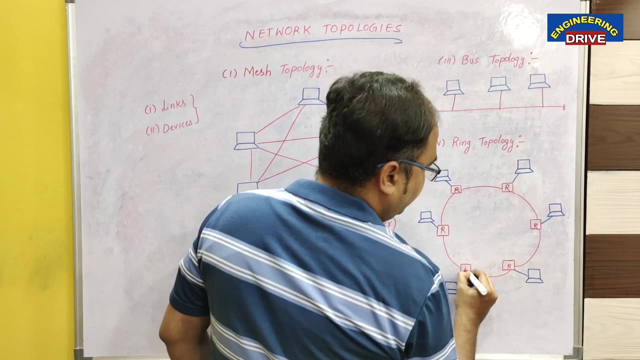 We can see here, this is a ring structure. Now, sir, in ring topologies, what is this box, sir, which you have taken here? These boxes, they are actually repeaters. So they are repeaters. So what is the job of repeaters Already? 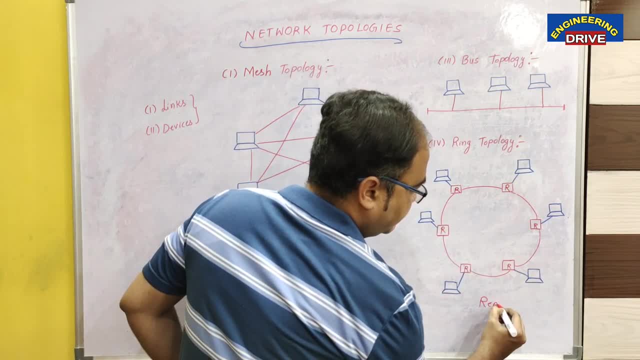 we have discussed this. So what is the job of repeaters? So what is the job of repeaters Already we have discussed in our previous videos. they are actually repeaters. Now what happened, How the communication will take place and what is the job of repeater. 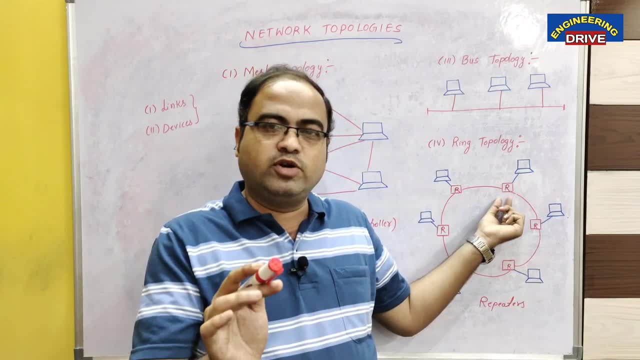 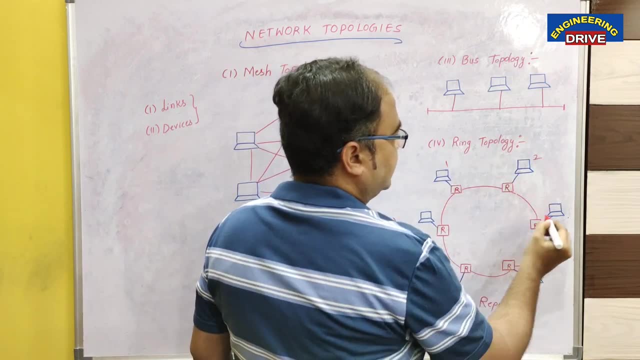 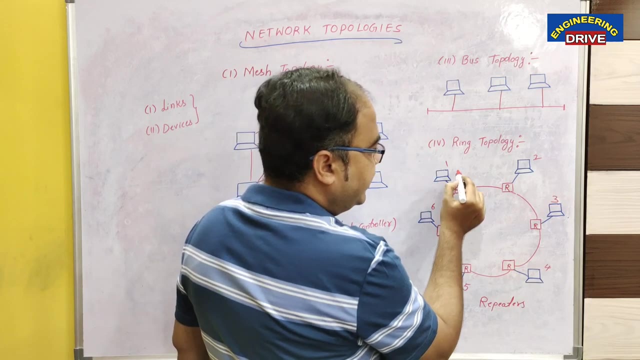 Why we are calling this device as a repeater. I will tell you now, Carefully, listen. Let us say if this is device number 1 and this is device number 2 and this is device number 3, 4, 5 and 6.. If device 1 want to communicate with device number 4.. 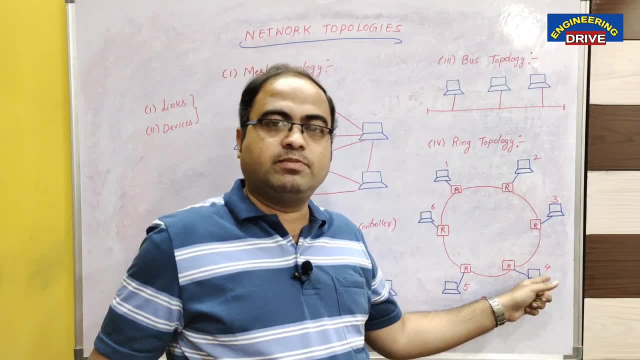 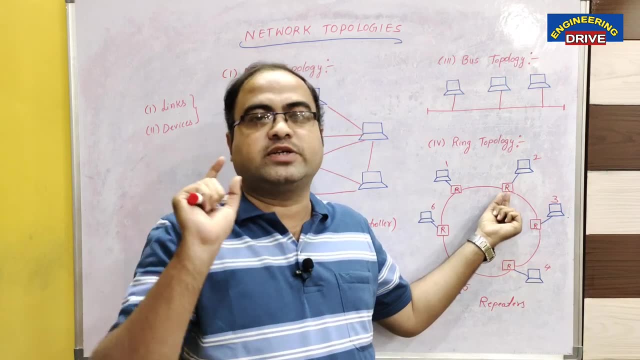 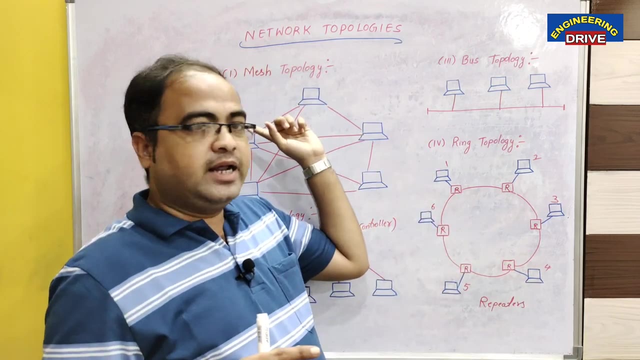 Device number 1 want to communicate with device number 4.. Then what happened? From device 1, the data will be transmitted to device number 2 first. It cannot be transmitted directly to device number 4 because there is no direct link available here, unlike mesh. 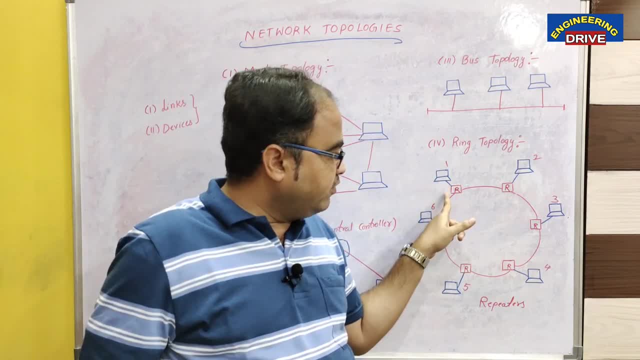 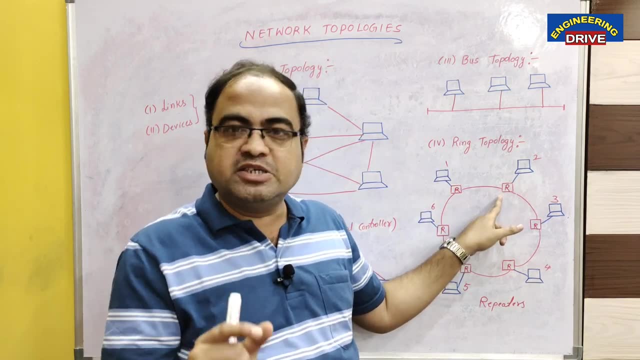 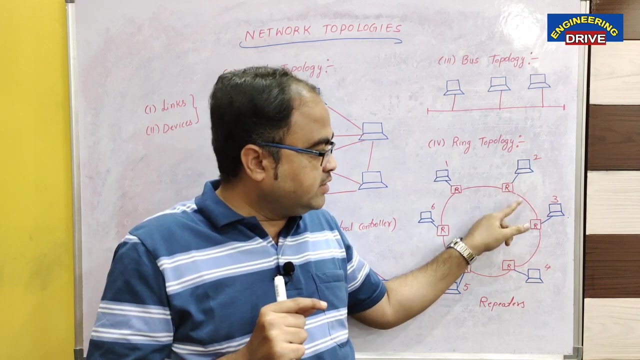 topologies. That is why what we will do here: From device number 1, the data will be transmitted to device number 2 first, And in device number 2, repeater is installed here. What this is This repeater will do. what this repeater will do: It will take this data and it will forward. 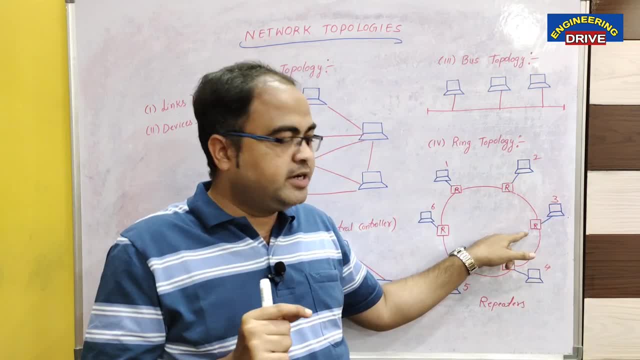 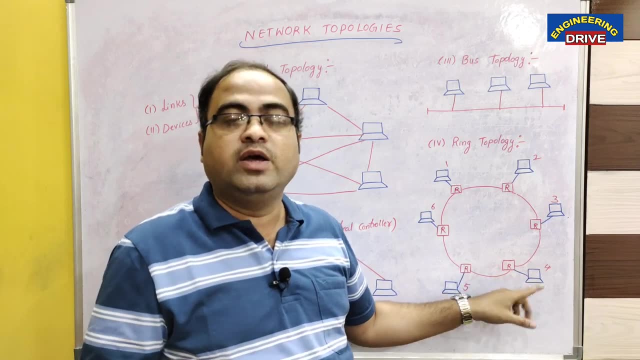 this data to device number 3.. And from device number 3, the repeater will do the same thing. As this data does not belong to device number 3, it will transmit the data to device number 4.. And finally, the data will reach to device number 4.. So, repeater, the job of a repeater. 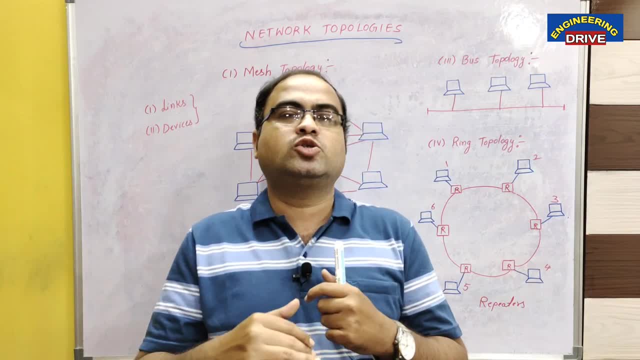 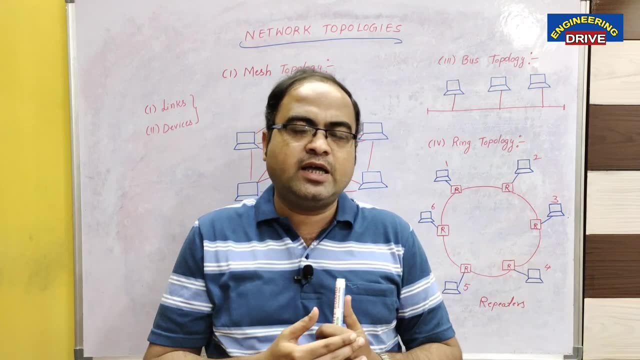 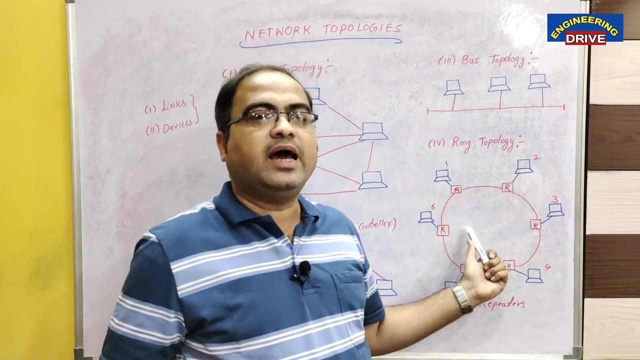 in networks is to amplify the signal and so that it can reach to longer distances. Here it is taking that particular data and it is transmitting the data to the required destination through longer distances. That is why we are calling these devices as repeaters, So dear.